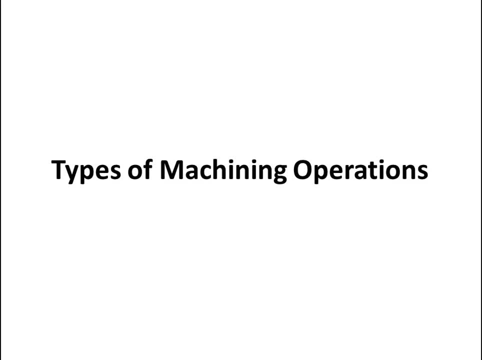 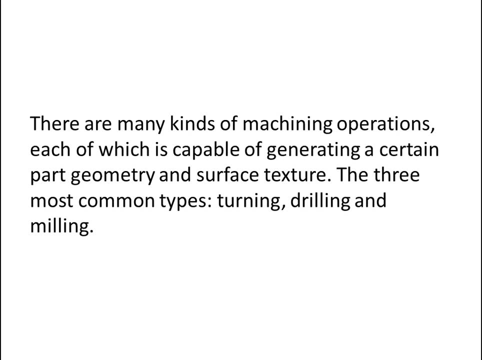 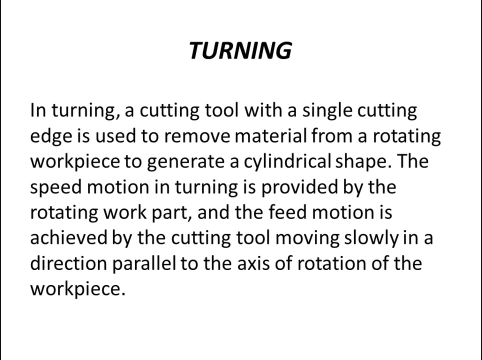 Let's talk about types of machining operations. Actually, there are many kinds of machining operations, Each of which is capable of generating a certain part: geometry and surface texture. The three most common types: turning, drilling and milling. Let's talk about turning In. 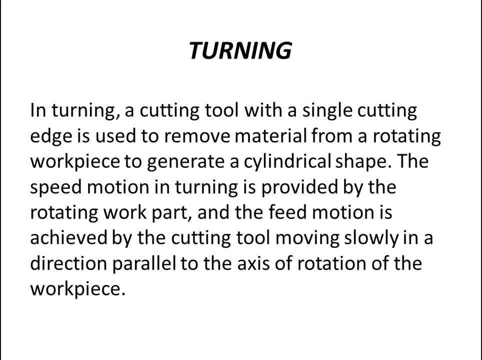 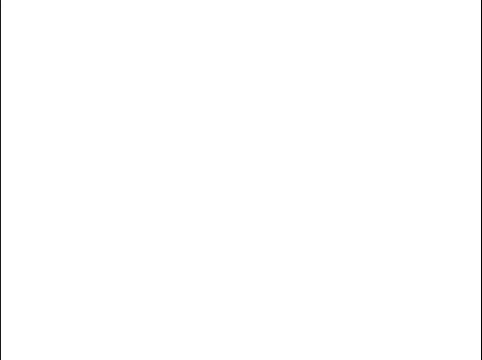 turning. a cutting tool with a single cutting edge is used to remove material from a rotating workpiece to generate a cylindrical shape. The speed motion in turning is provided by the rotating work part And the speed motion is achieved by the cutting tool moving slowly in a direction parallel to the axis of rotation of the workpiece. And there is a figure of: 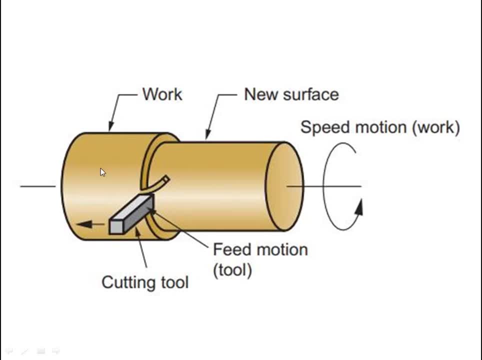 turning. So this is a work piece, This is our work And this is the cutting tool, And the work is rotating in anticlockwise direction. This is the direction of rotating And this is the speed motion of the tool. So, because of the rotation of the work and speed motion of the cutting tool, the material, 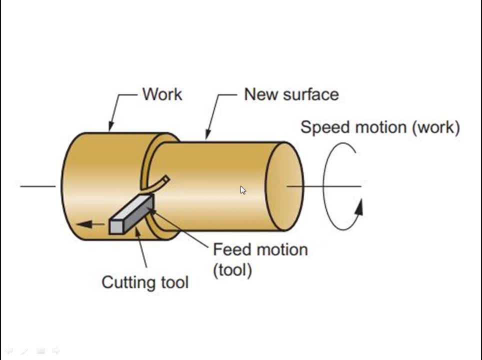 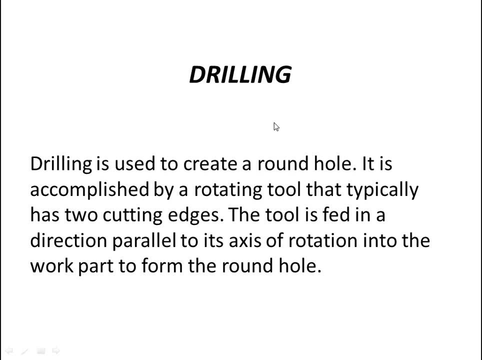 is removed from the work And finally, we get a new surface. And let's talk about drilling. Drilling is used to create a round hole. It is accompanied by rotating tool that typically has two cutting edges. This tool is spread in a rotation parallel. 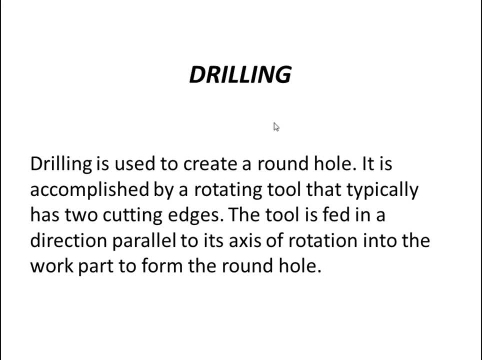 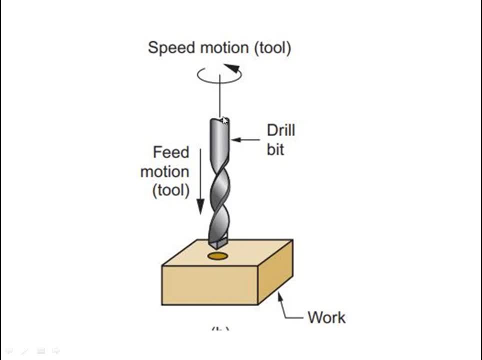 to its axis of rotation into the work parts to form the round hole And there is a figure of drilling. So this is the journey, And this is a drill spinning bit or cutting tool, And it is rotating in anticlockwise direction and this is a feed. motion, downward motion- of the tool, And this is the expression of the work piece, which is shown on the 30 Heinzel, which is also an automated sculpting system and where, by default, the work piece is not integrated directly into a solid object. However, it is directly connected. 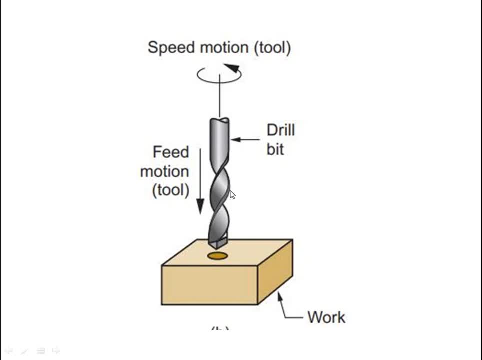 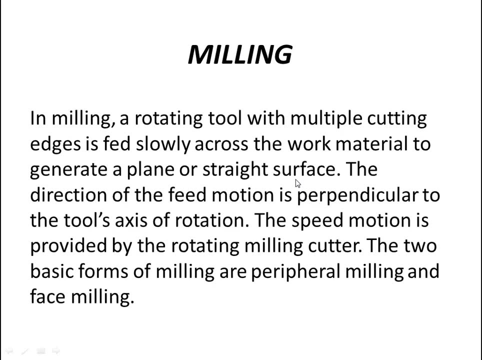 And because of the motion of this drill bit or cutting tool this hole is created. Let's talk about milling. In milling, a rotating tool with multiple cutting edges is fed slowly across the work material to generate a plane or straight surface. The direction of the feed motion is perpendicular to the tool's axis of rotation.